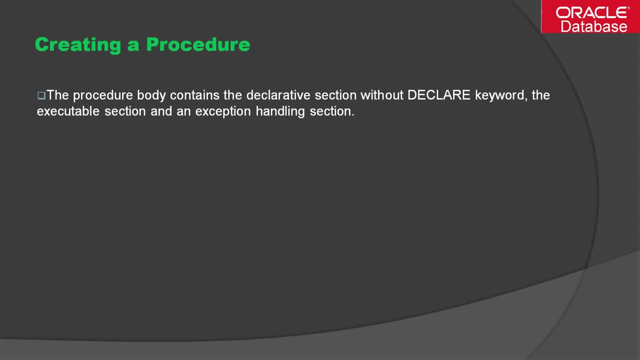 in this case we don't need to use the declare keyword. We can create a PL SQL block using the declarative section. If you create a stored procedure, so in declarative section you don't need to declare a- I mean declarative section- you cannot declare. you don't need to use. 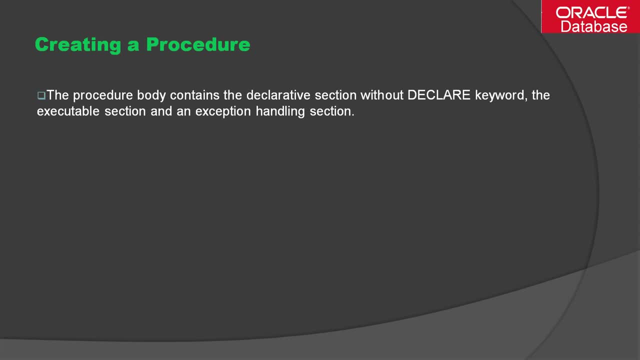 declare keyword right. Then you have executable section. means there you are going to write the business logic, all the SQL statement and all, And finally you can have a exception handling code as well. Yeah, Now this is the basically general syntax. how to create procedures. First, 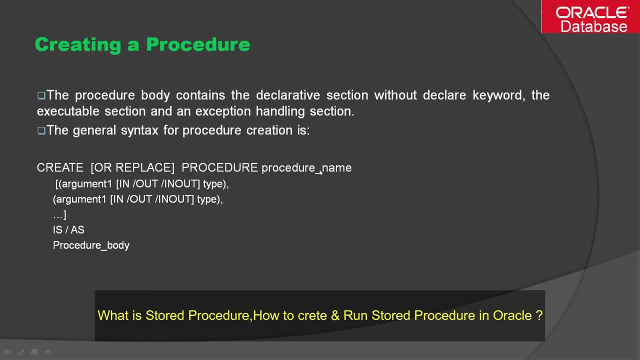 of all you have to write create Procedure, procedure name. And here you can write like this: create or replace. If already a procedure is existing with this name, whatever name you have provided, then existing procedure will be dropped and recreated again. right? If you do not specify or replace, simply you write. 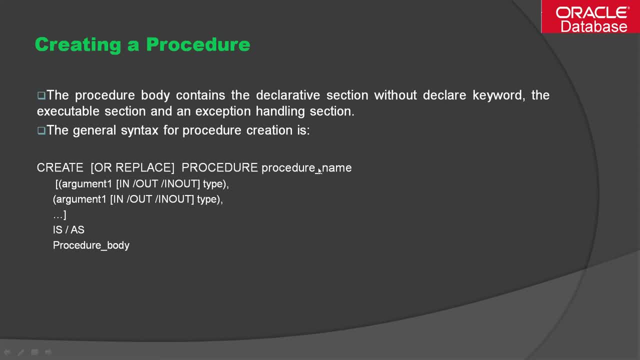 create procedure procedure name. If procedure is already existing with this name, then you'll get an error right Now we have to specify: if you have some input parameter or output parameter, those parameter you have to specify In this bracket parenthesis, right? If you do not have, then you don't need to simply. 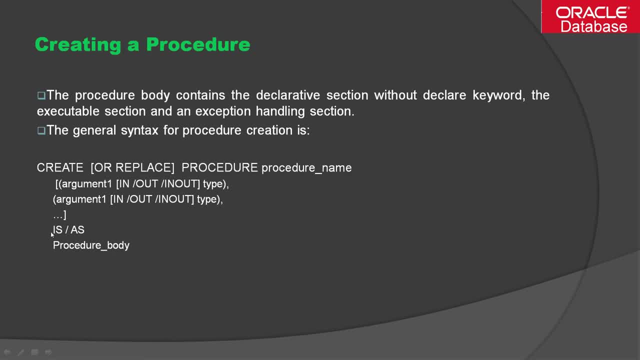 specify a procedure name would be enough. After that you have to specify either is or as right Keyword And after that you have a procedure body right In procedure body. basically, you have three sections: declarative section, then executable section and exception. 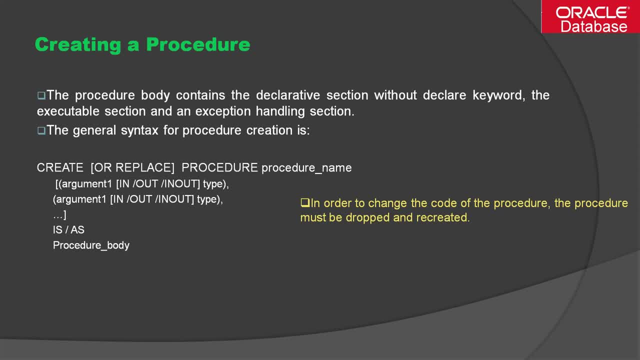 handling section. Yeah, So there are some key points you will have to keep in mind in order to change the code of the procedure. The procedure must be dropped and recreated, right, If you have already existing procedure, if you do some modification, then you have to recreate the. you have to drop first of. 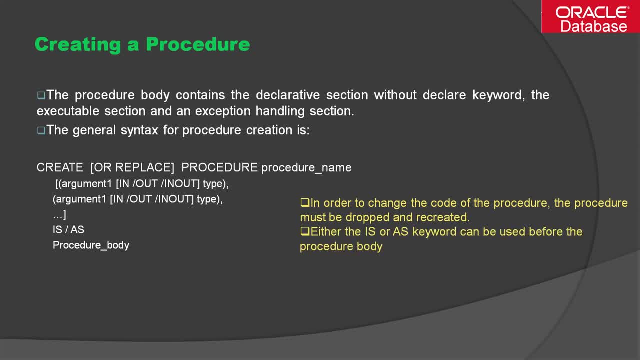 all and then recreate the stored procedure. Either the is or as keyword can be used before the procedure body, right? So before the procedure body, either you have to use is or as keyboard. Now here is the, basically a stored procedure, Basically snippet what I have shown over here. 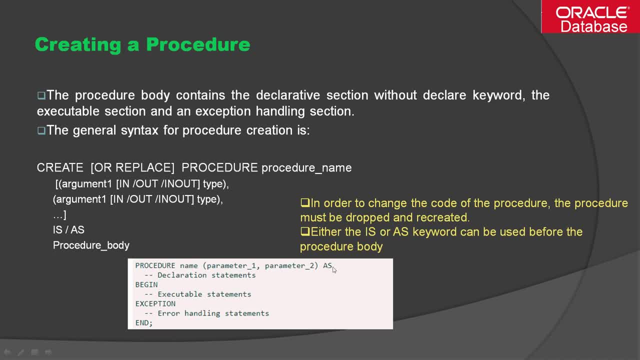 the procedure, then name, then parameter- you can specify after that is. or as keyword you can specify. then you have begin and end. Between the begin and end you can have executable statements, then exception handling code as well. right Now some of the key points always. 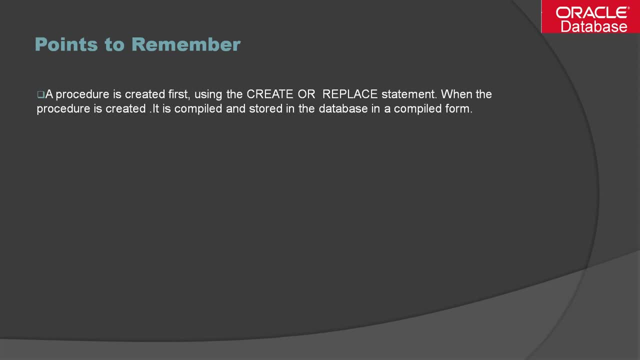 you have to keep in mind like a procedure is created first using the create or replace statement. When the procedure is created it is compiled and stored in the database in compiled form. So once you create the stored procedure, then various developer can call. 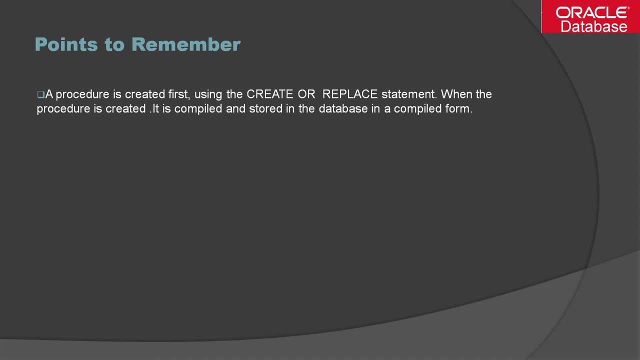 that stored procedure. right? That's the advantage of a stored procedure: that gets compiled and stored on the database. Now, when procedure is called, the parameters can be passed. It is not compulsory to create a procedure which accepts parameters. If created, then it must. 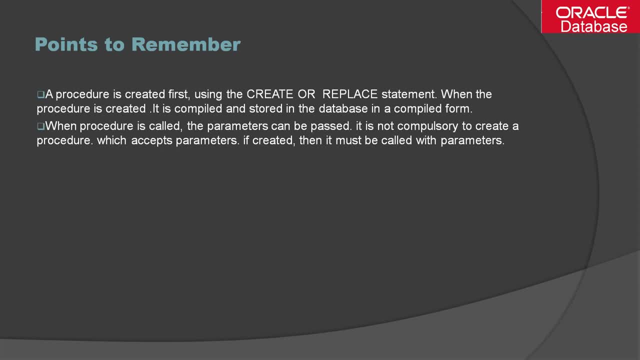 be called with parameters, So you can create a stored procedure with or without parameter. If procedure is created with parameter, then you have to pass those parameters to invoke that procedure. Yeah, Now procedure. procedure call is a PLC call statement in itself. When procedure is called, the control passes through the executable. 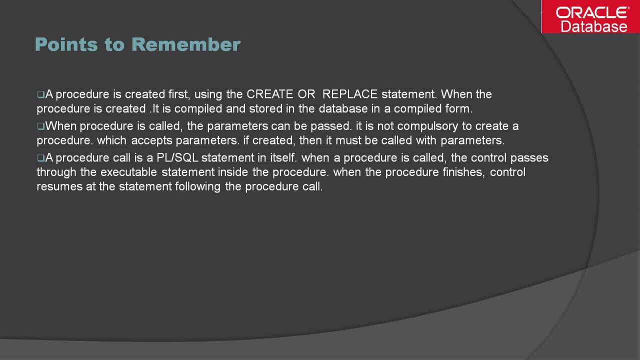 statement inside the procedure. When the procedure finishes, control resumes at the statement following the procedure: call right, So from PL SQL block. if you call the procedure right, then call will be transferred to the executable statement inside the procedure Once procedure. 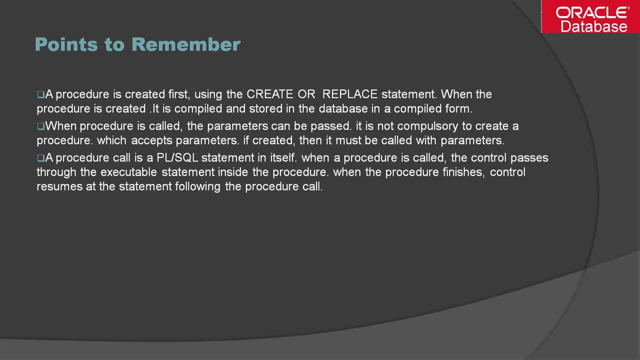 finishes the call, then control control will return to the statement from where it was called, From where you have called the stored procedure. right Now, a procedure is a PLC call block with declarative section without declare keyword. Already we have discussed an executable section and exception handling section. Yeah, So this is all about the concept. 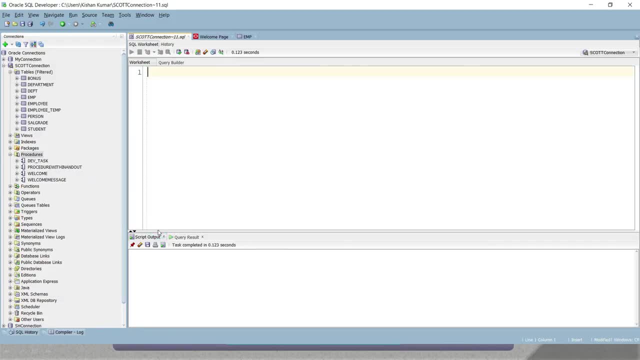 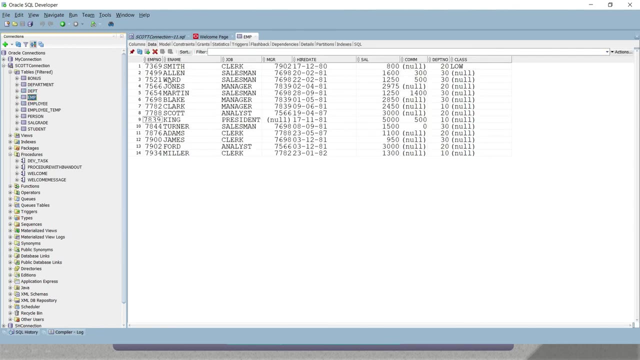 related to a stored procedure. But now let's move towards to create a simple stored procedure so that we can have a better understanding. So here, if you look into the employee table, so employee table you have, you have employee salary here. 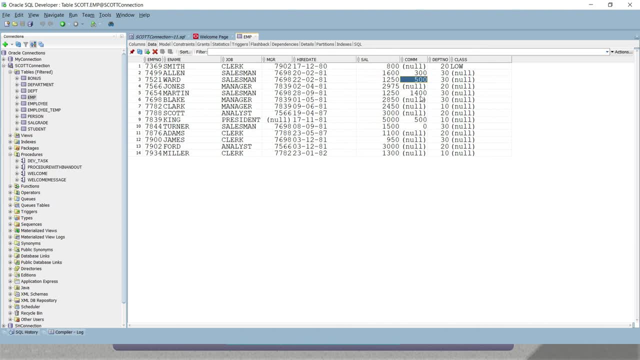 Right. So just I would like to create a stored procedure which will return employees total salary. When I say employee total salary means a salary plus commission. that would be total salary or total compensation right, And employee number would be the input parameter. 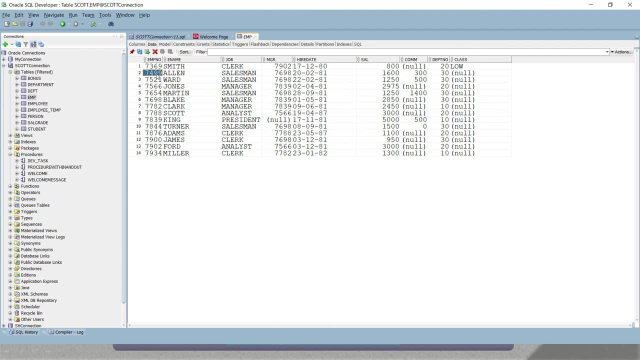 I hope you understood. I would like to create a procedure which basically takes employee number as an input and that will print employee total commission in the employee table, So total compensation or total salary, and that will be calculated by salary plus compensation. if salary is null, then null should be replaced with the zero and that should be added into the salary. 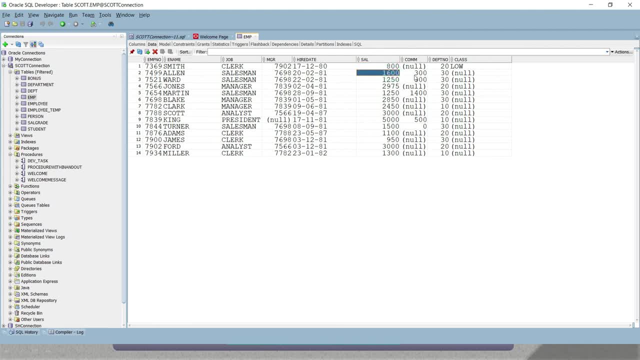 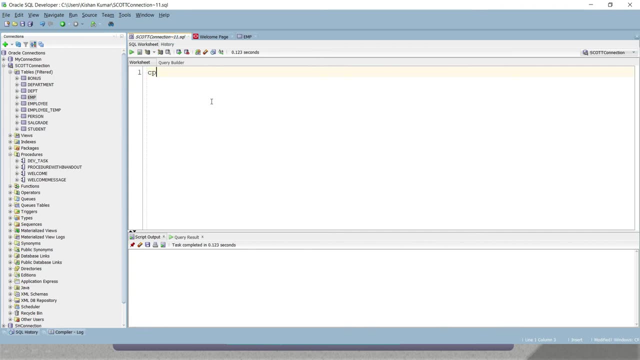 so 800 plus 0, 800, 1600 plus 300, 1900, something like should be the output. right? so here to create a stored procedure, i'm going to write cp. cp is nothing but the. this is: this is a shortcut to create a stored procedure snippet, right? so this is the stored procedure snippet. 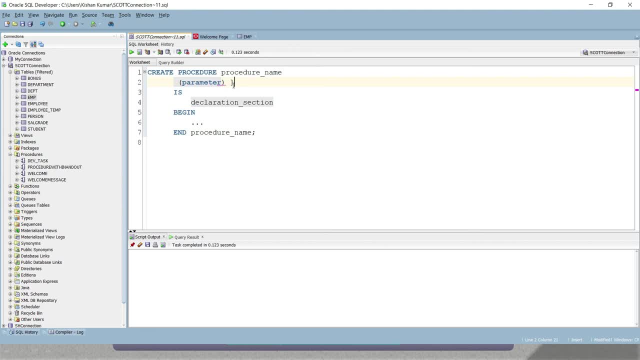 here we have one in this bracket, this, this, this one you can remove. here i'm going to declare some basically input parameter. so here input parameter would be employee number, so i would write emp underscore number, right. and here this is a input parameter, so optionally you can write in keyword, right. 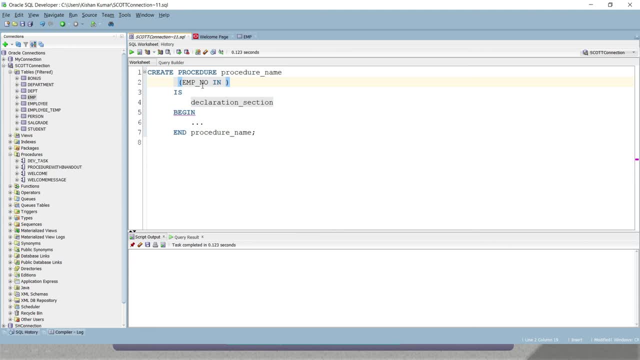 so in out and in out. there are three modes of uh: store or stored procedure of functions, uh input output parameter. so here in is optional, in is the default one. in you can write. you cannot write that. that is also possible. you can leave it in. if you do not provide the in that, this will be considered. 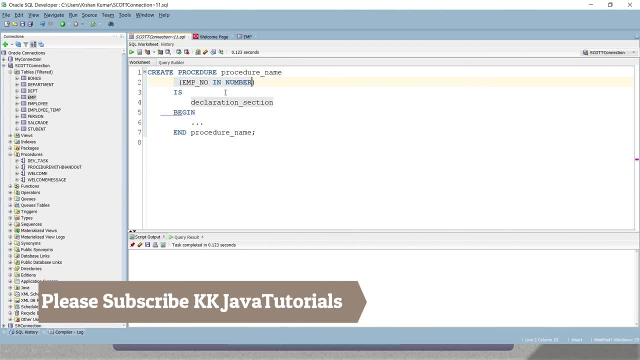 as input parameter here data type you have to write. so here here employee number is an input parameter. that's why i have written in: this is optional, you can leave it, not a problem at all, but i'm going to write in and number is the data type, right? so implied number i'm taking as input. 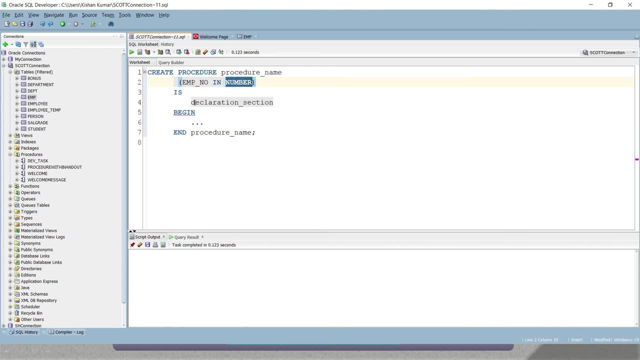 parameter, which is type, type of number. now here i'm going to. this is the declaration declaration section. after that you can write is or as right. both will work. after that, this is declarative section. declarative section is optional. but here i'm going to declare one variable like: 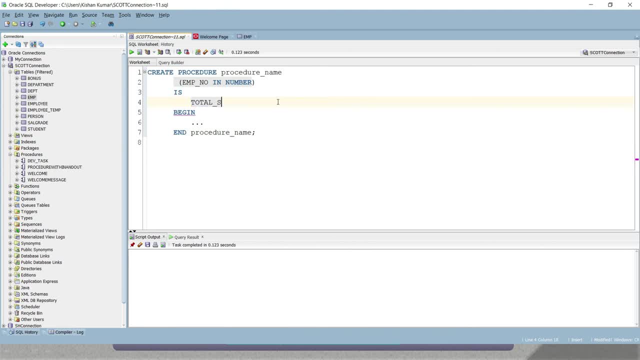 i would say total salary. so this variable i'm going to use in my uh store procedure, this body. so before that we need to declare this one. this is type of number. i'm going to write 7 comma 2.. so so 7 is the total number of. 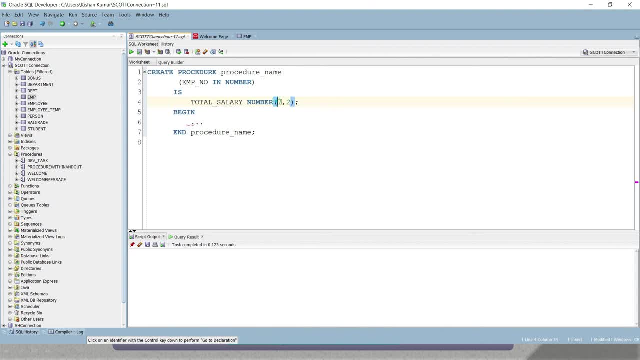 digits and 2 is the digit after decimal, right? so that's the meaning of this. now, here i'm going to write a sql query and here you have to give the basically stored procedure name. so i'm going to write: get, uh, get uh, employee- employee total salary by employee number, something like this, right? so this is store procedure name. 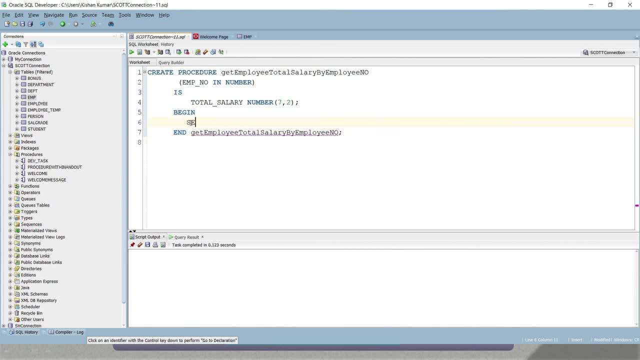 you have to put it over here as well, right, and here i'm going to write select. and here i'm going to write uh, basically salary plus nvl. i'm going to write, i'm going to use your function is called nvl. this is commission, one of the column, and here i'm going to add zero. 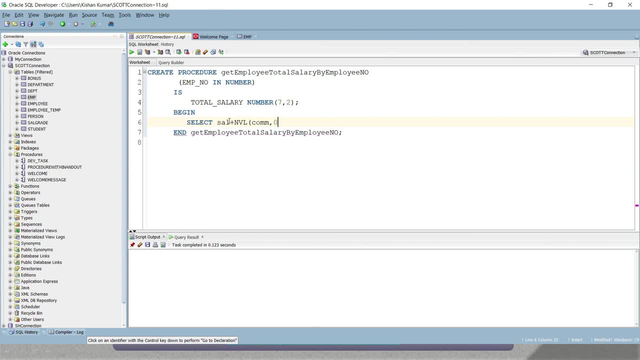 what's the meaning of this? just, i would like to add salary in commission, but to call to get the value of commission, i have used nvl function in bl function. first of all i have used a nvl function, and then i would like to add salary, which is zero, and then i would like to add salary in commission. 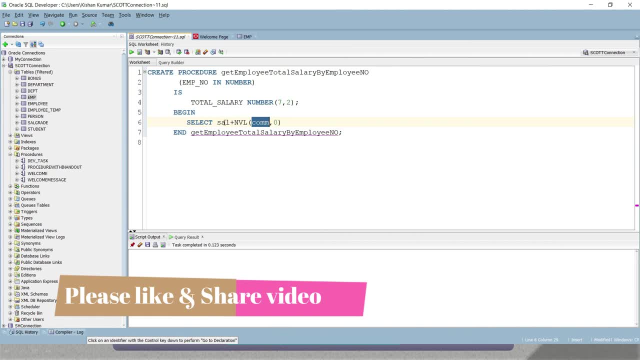 look into this column. if this column value is not null, then that that will be added into the salary. if column value is null, then this will replace null with zero. that's the meaning. so i just select salary plus nvl, commission, comma, zero into this. declare variable right. so this calculated value. 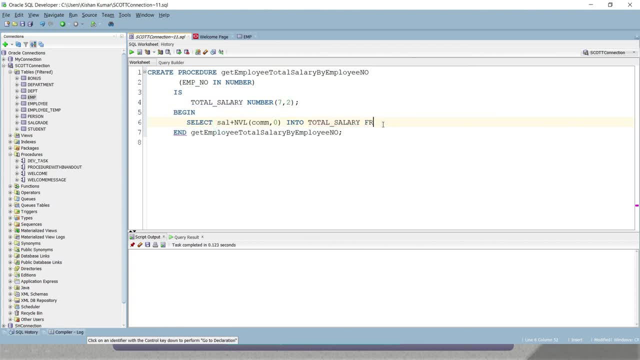 just, i'm going to store in this variable right, i would say from emp, where employee number, emp number equals to whatever input is coming from the client. that's right now, here these things. i am going to print it over here. so i would say: dbms underscore output. 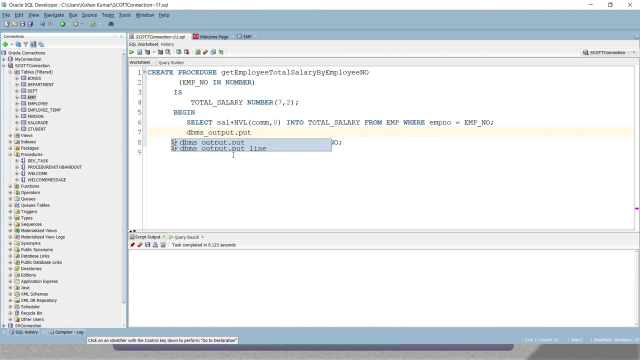 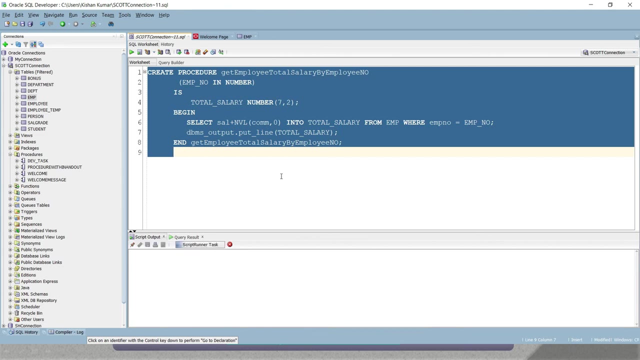 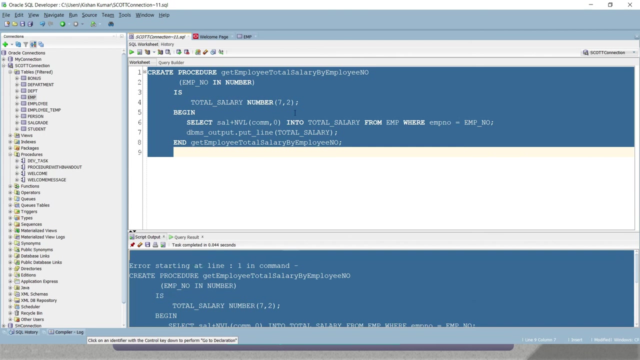 dot, put line, and here i'm going to print this total salary. very simple store procedure. i have written: yeah, now i'm going to basically run this store procedure now saying that some error has occurred, saying that identifier is too long. so i think this is what procedure is: saying that too long? i think so i'd say, i'd say get. 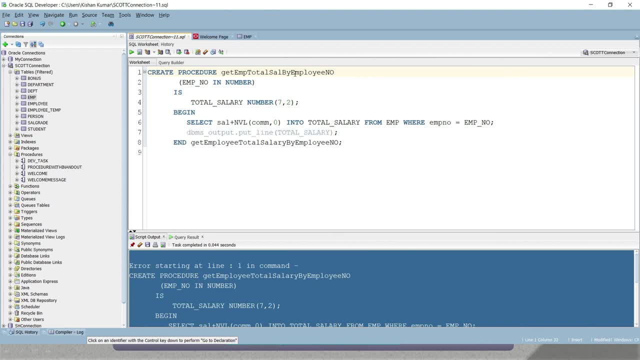 emp cell by emp number. yeah, this same you have to replace here and here you can write: if you refresh this one, then if you procedure is not created it right, so no problem with this one. if you refresh this one, then if you procedure has not created it right, so no problem. now keep on writing. this procedure will help with the process. 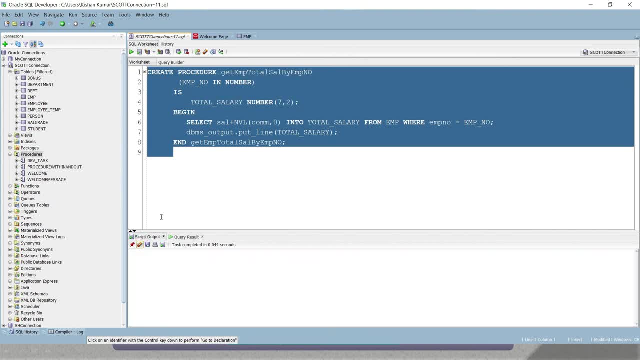 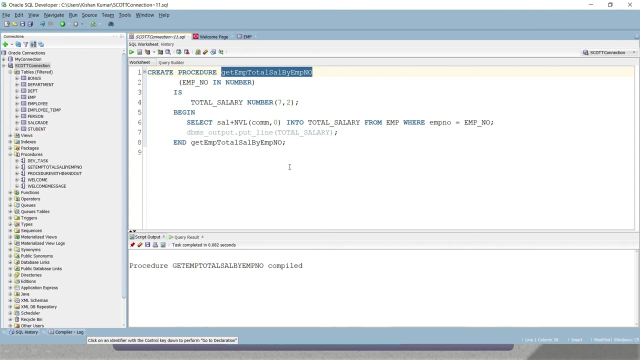 then run it again. so let me clean this terminal. say that procedure is compiled means this procedure is created. now let me refresh. so here you can see this stored procedure has been created. now let's call it. so how we can call it? to call it you have to write execute right, and here you have to pass the employee. 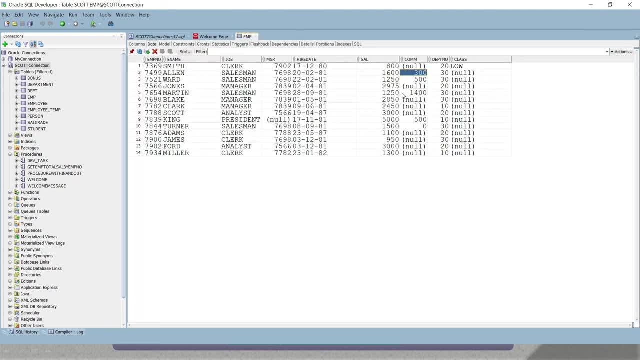 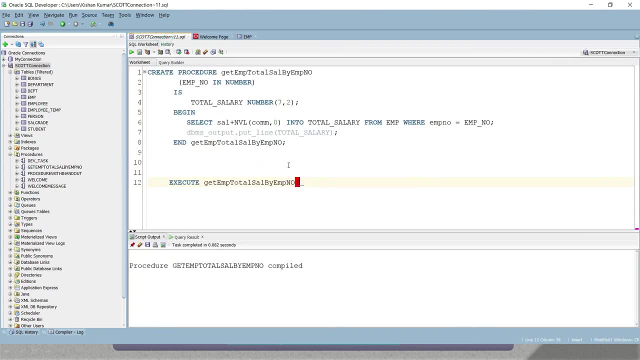 number. so let's say I would like to calculate salary for this guy right, whose employee 7654? yeah, 7654, I am passing. and here to get the output from DBMS output, I am going to write set server output on so that DBMS output. 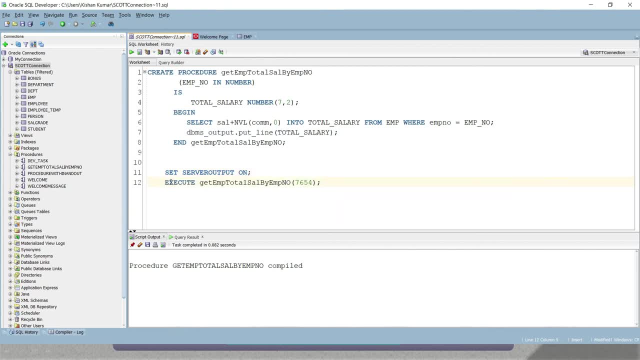 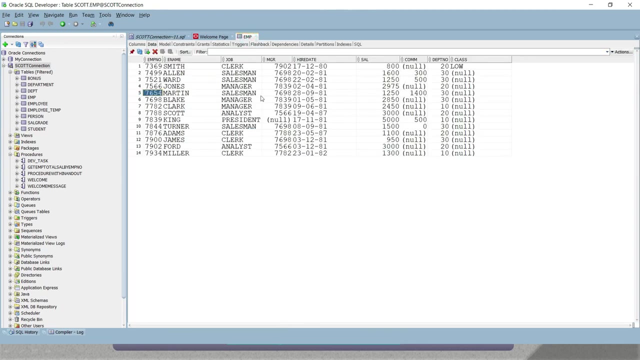 will work as there is possibility will not get output from DBMS output. what we have written to assume procedure to enable is just: I have written this: if I execute this one, then here you can see 2650. that's the total salary of the employee, right? so if you look at this guy, this guy has salaries. 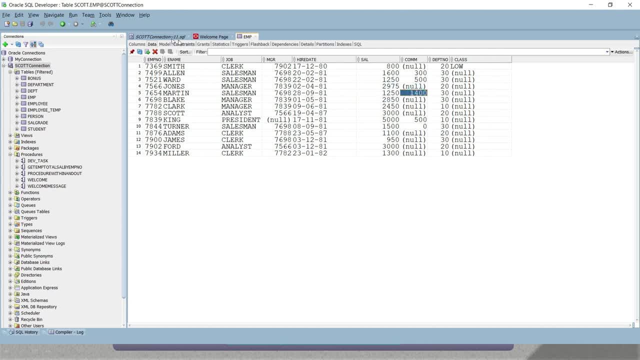 1250 and this is the Commission. if you add both, then this will come to six five zero. that's the final output. let's say I'm going to calculate salary for this guy whose Commission is null right, whose name is a Smith right, whose employee is: